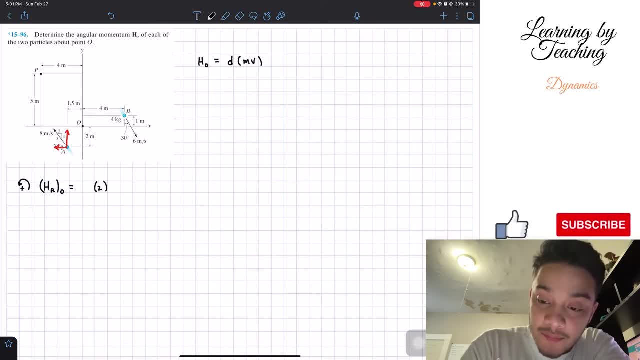 So we're going to have two meters multiplied by the mass, which is three kilograms, As I mentioned before, multiplied by its velocity- Well, it's x component of this velocity- Well, its magnitude is eight. but we have three out of five going in that direction. 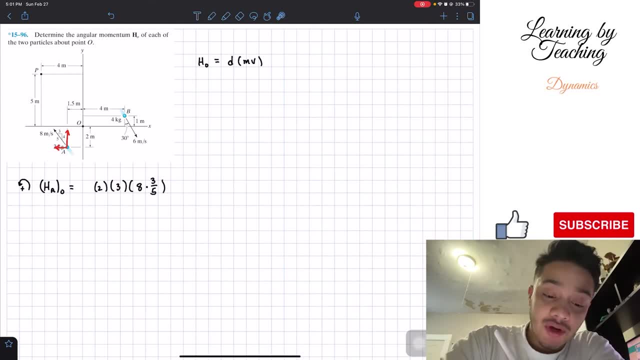 Okay. Now the last thing that we need to know is that, since I'm interested about this 0.0.. Okay, And the velocity is going this way, my momentum will want to go clockwise direction. Therefore, it's going to be negative. 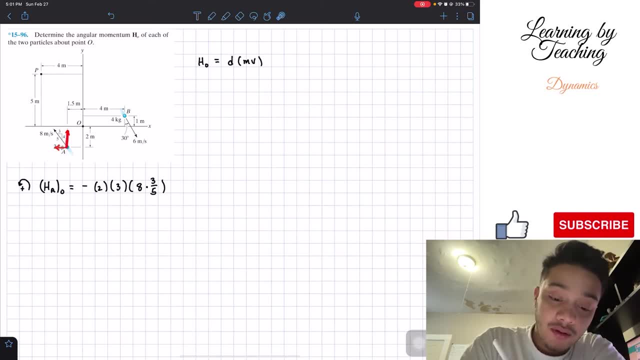 Then we're going to do the same thing, but with my y component of my velocity, And same thing is going to go clockwise direction. So it's going to be negative. Its distance is going to be marked by this 1.5 meters. 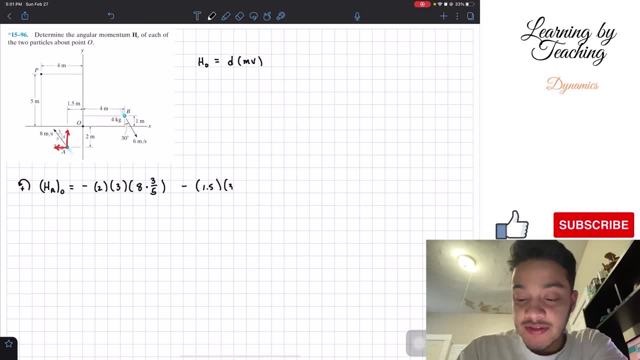 So we got 1.5 multiplied by the mass. The mass stays the same, equal to three, And its velocity is going to be eight multiplied by four over five. Very similar. If we plug this into our calculator, we will find out that this is equal to 57.6.. 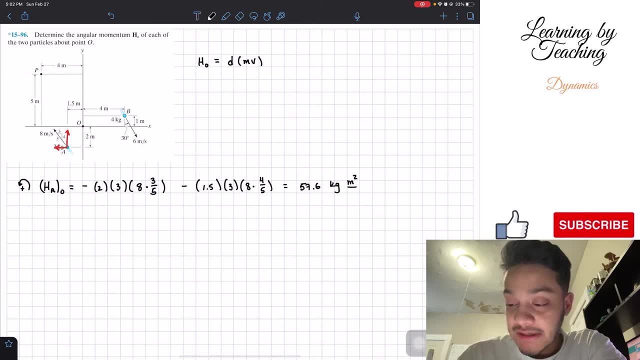 And the units is going to be kilograms, meter square per second. Okay, So we're done with our particle A. We're going to go ahead and now concentrate my particle B. We're going to break it very similarly Into its y component and its x component. 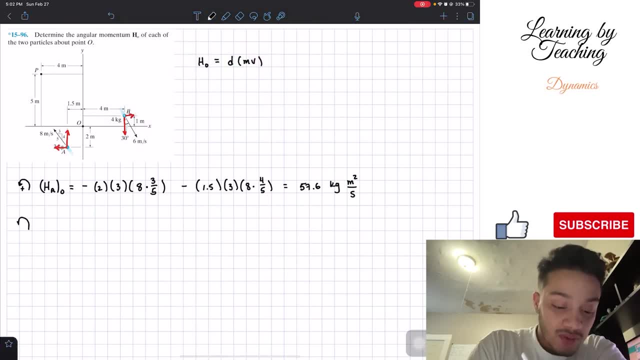 Okay. So again, we're going to assume counterclockwise is going to be positive And we're going to do the angular momentum particle B around my point O. And what do we have? Well, let's start with the x component. 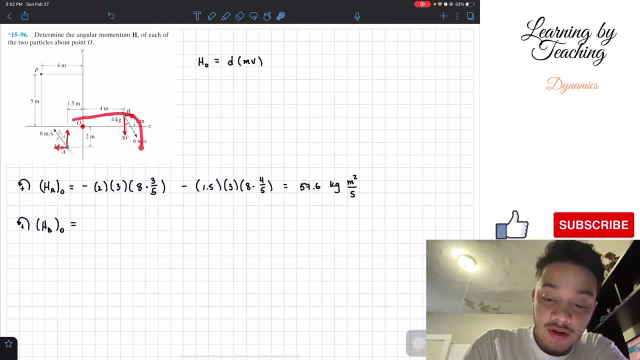 Well, the x component, if I'm holding here and I'm going around this velocity, we will create a negative value. The distance is one meter, as we can see here. One meter multiplied by its mass, which is four kilograms, multiplied by its velocity. 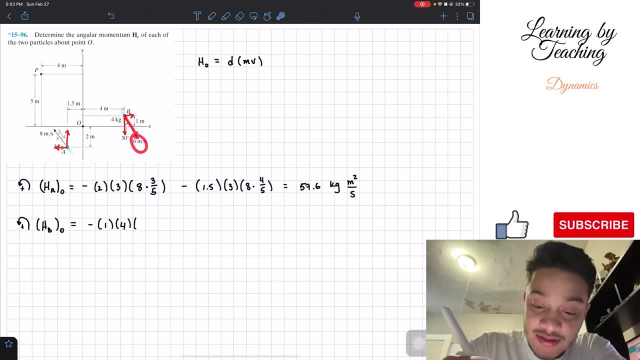 Well, the magnitude of this entire velocity is six, But how much of it is going to be its x component? Well, it's going to be the magnitude six multiplied by the sine of 30 degrees. Okay, Then we're going to do the same thing for its y component.